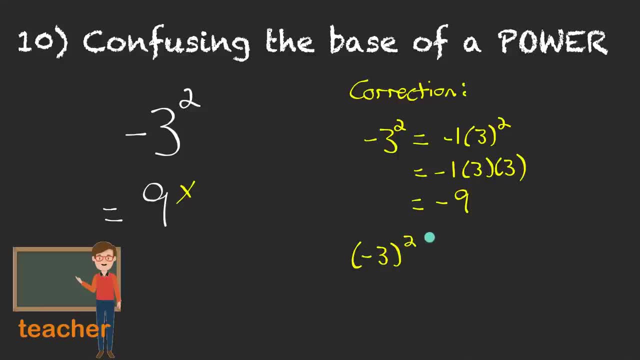 written like this: negative three in brackets squared. that would mean the base of the power is negative three, which means we have negative three times negative three and that is positive nine. So make sure you know the answer. Thank you, So you know this is not the same thing as this. Pay attention to what the base of the power. 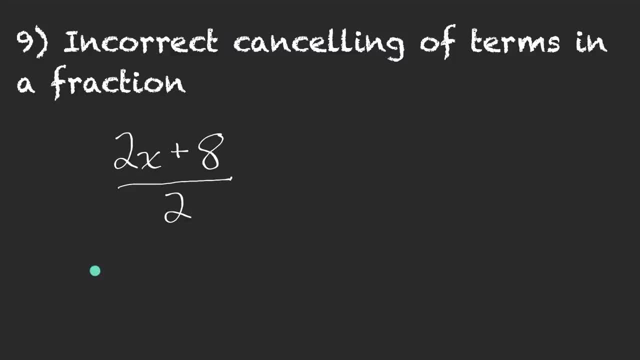 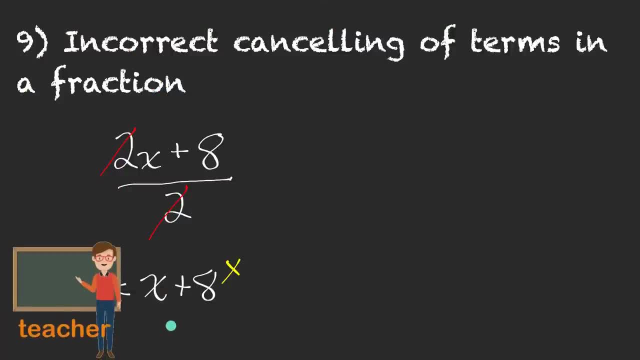 No, sorry, that's not correct, But this is actually a super common mistake- to actually forget to divide both of the terms by the denominator. You need to divide the 8 by 2 as well. Let me show you how to do that. Okay, one way you could do this so that you don't. 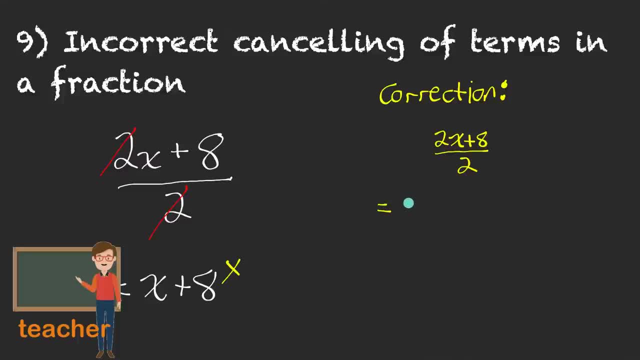 make that mistake would be to separate this into two fractions being added. Since the 2x and the 8 are both being divided by 2, I could separate this into 2x over 2 plus 8 over 2,, which is x plus 4.. Notice, the 2x and the 8 are both being divided by 2.. Another: 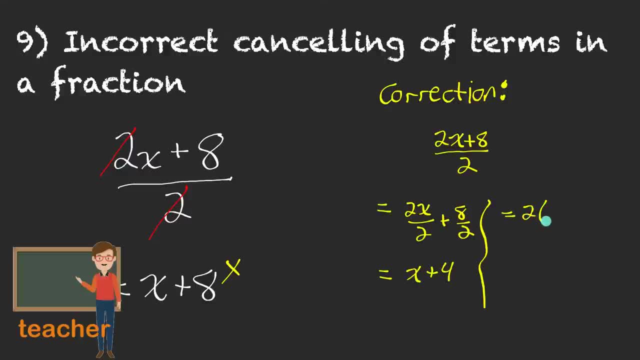 way you could do this. I could common factor a 2 from the numerator, giving me 2 times x plus 4, all over 2.. And now that the numerator is in factored form, you can look to cancel or reduce factors with each other. So I see a factor of 2 in the numerator, a factor of 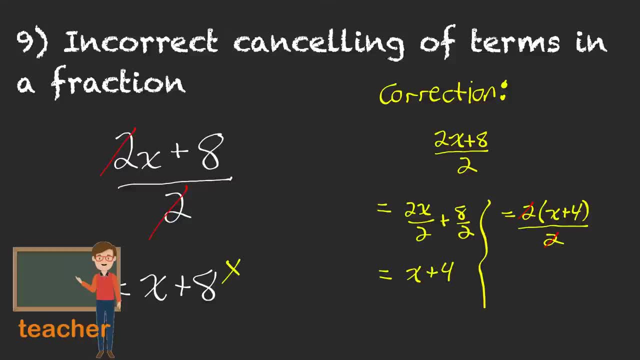 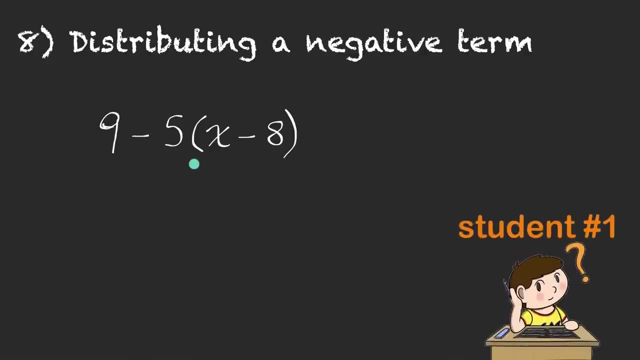 2 in the denominator. something divided by itself is 1, so I can cancel those out And I'm left with just x plus 4.. So two different ways to think about getting that same correct answer. but x plus 8, no Okay, I just need to simplify this. I remember distributive. 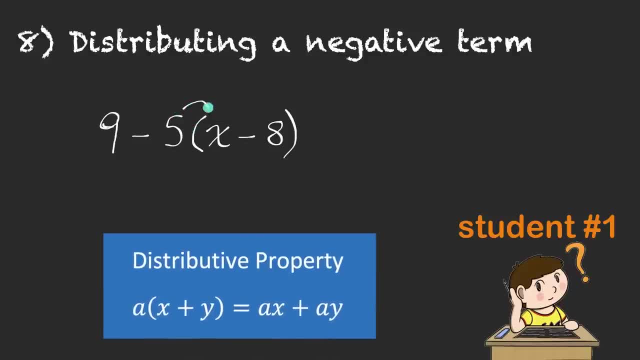 property. I know. you just take whatever is in front of the brackets and multiply it by everything in the brackets and then the brackets are gone. So I've got this 9, I'll leave that there minus. and then I have to do 5 times x, that's 5x, and 5 times negative 8, that's. 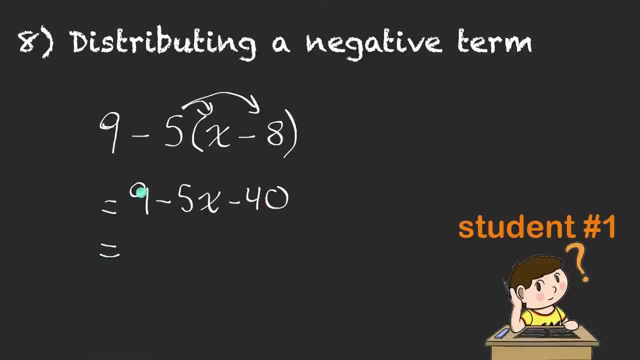 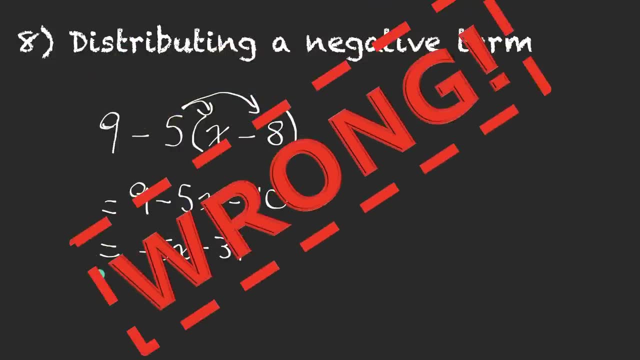 negative 40. And then I can collect my like terms: 9 minus 40 is negative 31,. so I've got negative 5x minus 31.. Alright, to start this one. I'm just going to start collecting some like terms. I've 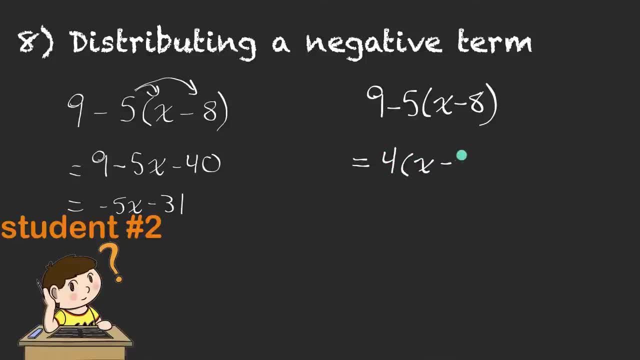 got a 9 minus 5, that's 4.. It's going to be easier if I do that first, And now I'll distribute the 4 in. I've got 4x and then minus 4 times 8, that's 32.. Nice. 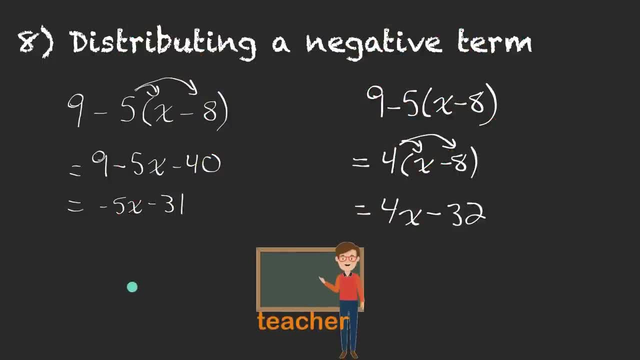 Okay, both of you actually just made one small mistake having to do with orders of operations. Let's correct them. Student number 1 over here on the left, you shouldn't have just distributed the 5.. You should have distributed a negative 5 if you were wanting to get rid. 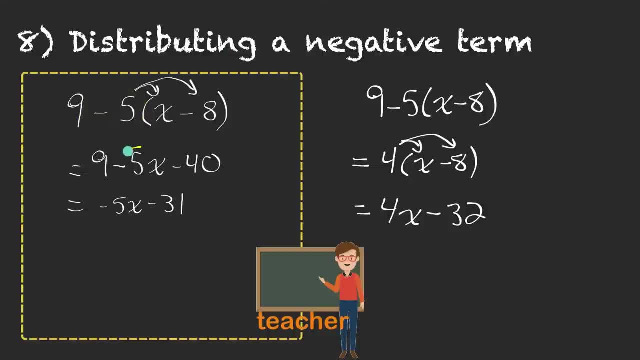 of the brackets all at once. If you did it the way you did it, this product would still have to be in brackets and you'd have to remember to subtract both of these, making this constant term wrong. We'd be subtracting negative 40,, which means we're going to have a negative 5.. So we're going to have a negative 5, and then we're going to have a negative 5.. So we're going to have a negative 5, and then we're going to have a negative 5.. So we're. 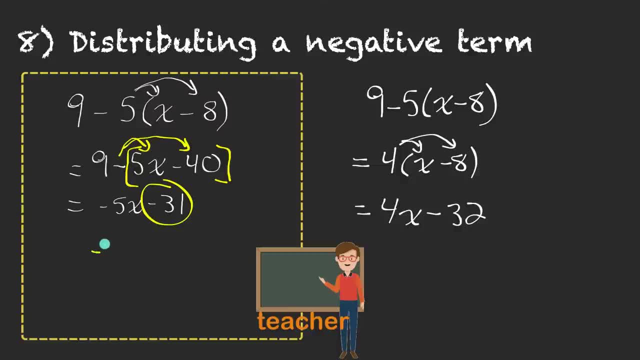 going to have a negative 5,, which means plus 40, so you'd have 9 plus 40,, which is 49. So you'd have negative 5x plus 49,, not negative 5x minus 31.. But that's not even how I would. 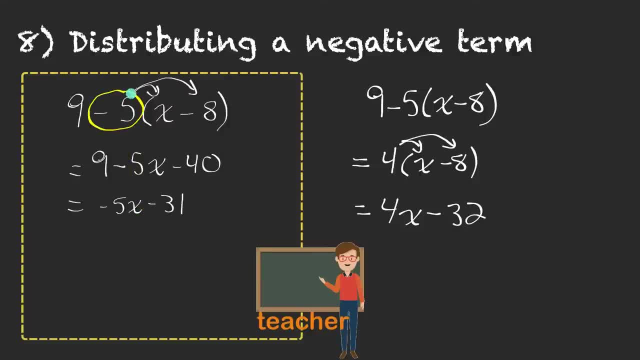 do this question. Like I said, I would distribute the negative 5, and then that would allow me to get rid of the brackets all in one step. So you'd have 9, and then negative 5 times x is negative 5x, and negative 5 times negative 8 is positive 40. So when you collect your 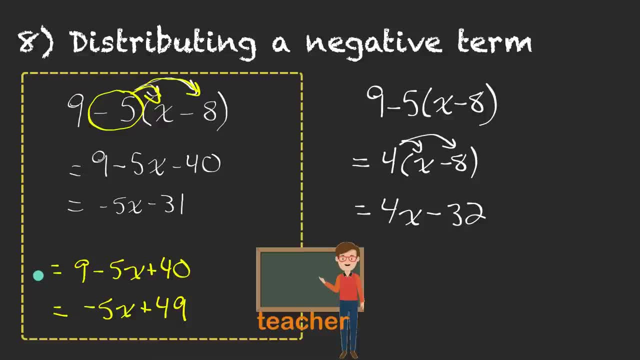 like terms. like I said, you'd have negative 5x plus 49.. All right, what happened over here, Okay? so yeah, this student didn't follow the correct order of operations. We can't do a subtraction first. This negative 5 is being multiplied. 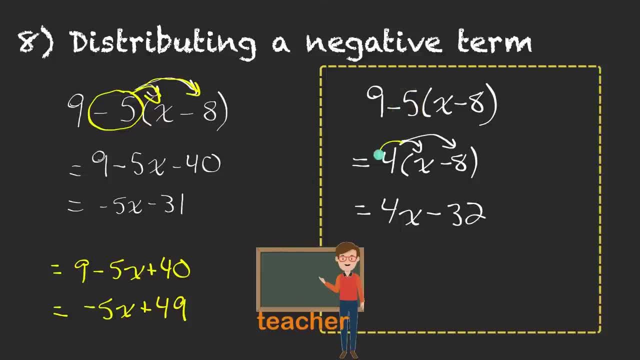 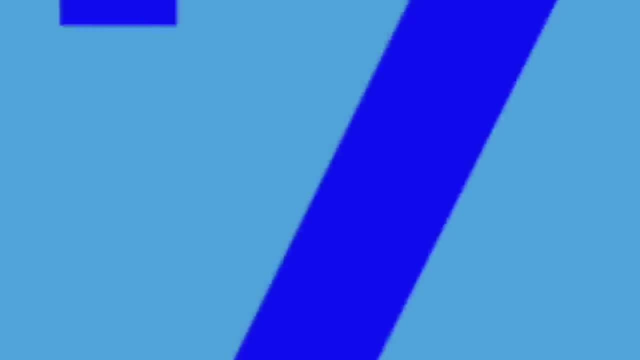 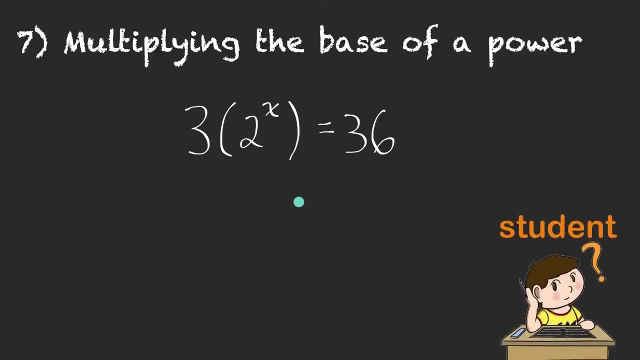 by something. so we'd have to do the multiplication before the subtraction. So no, right away. I know the answer's going to be wrong because they didn't follow the correct order of operations. Always remember bed mass, Ooh. exponential equations: These ones are always tricky for me. Okay, I think, Oh. 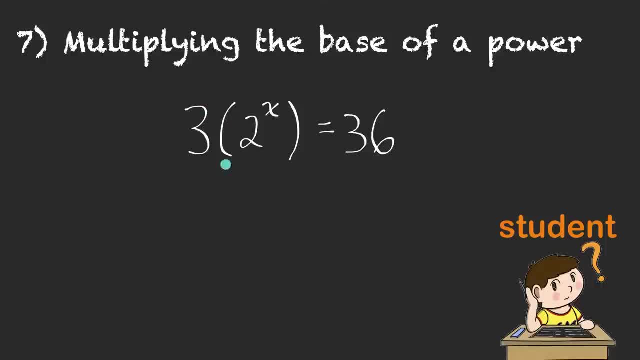 this one's actually pretty easy. I can do this one right: 3 times 2, that's just 6.. So I've got 6 to the x equals 36. And I know my powers of 6.. 6 squared is 36.. So my answer: 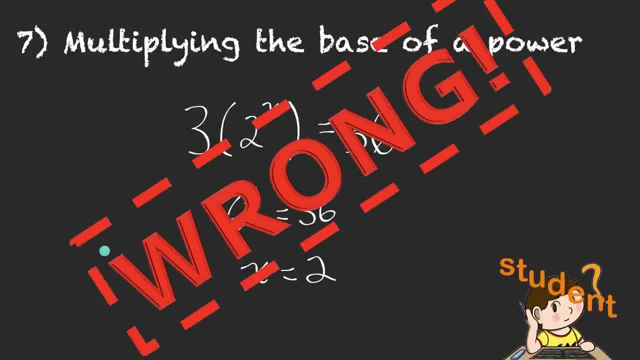 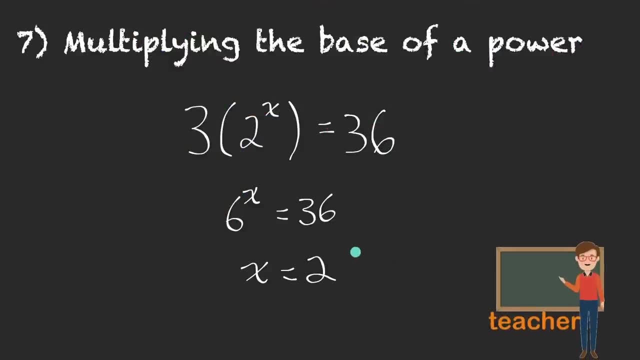 has got to be 2.. Before I show you where the mistake in this question is, let me remind you that when solving equations, you can always check to see if your answer is right or wrong. by plugging it into the original equation, I'd have 3 times 2 squared. Does that equal 36?? Well, 2 squared's 4.. 3 times 4. And 3. 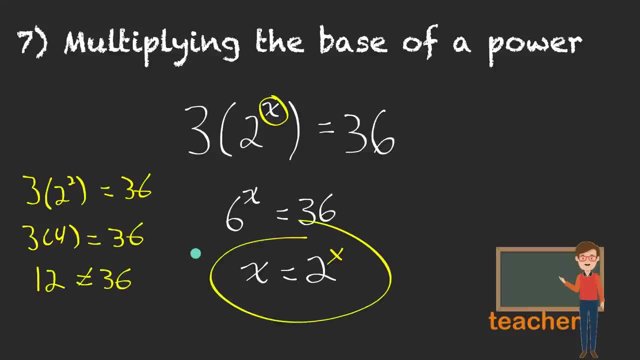 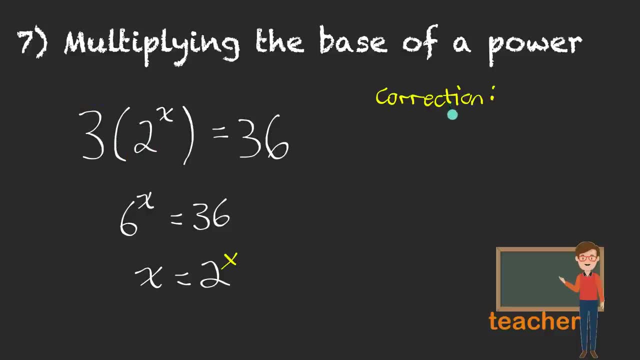 times 4 is 12.. Uh, 12's not 36.. So that shows you it's not the right answer. But what did you do wrong? You can't multiply the base of a power by a constant. That's not how it works. So what we would have to? 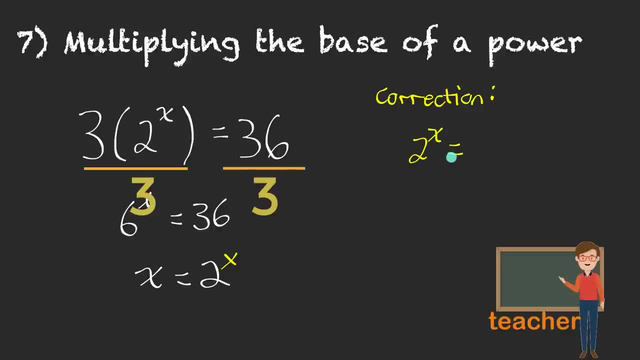 do to solve this question is divide both sides by 3 to start off with. So I'd have: 2 to the power of x equals 36 over 3, which is 36. 12. And really what we're looking for is what exponent goes on 2 to get 12.. And logarithmic. 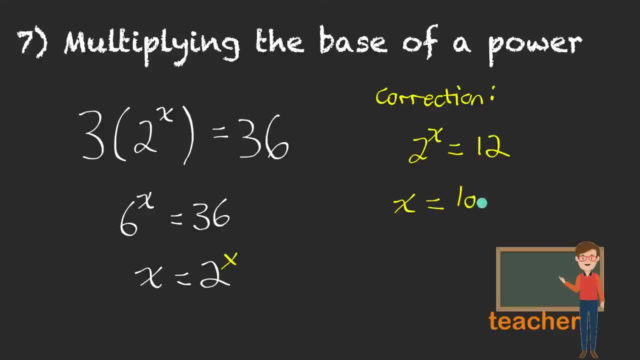 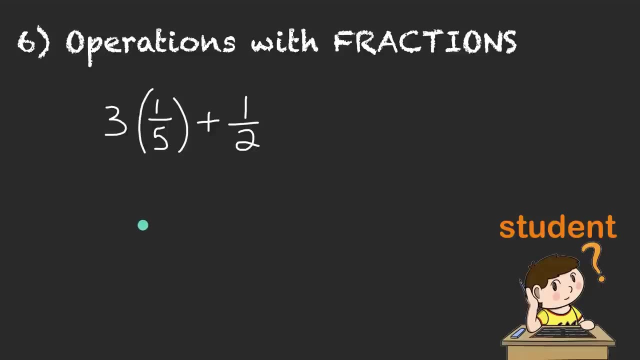 functions can find us missing exponents. The exponent would equal log base 2 of 12. And you can get an approximate value for that if you wanted, but that's the exponent that would satisfy this equation. Okay, fractions are sometimes tricky to remember all these rules, But, um, okay, I think the 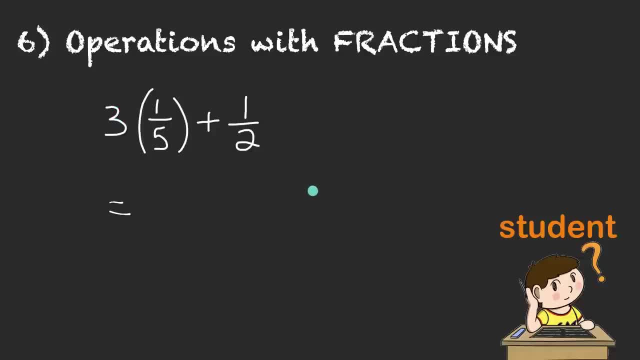 first. So bed mass: I have to do the multiplying first, So I'm going to multiply. okay, I have to do 3 times a fifth. Okay, 3 times 1 is 3.. 3 times 5 is 15.. Okay, that looks good. 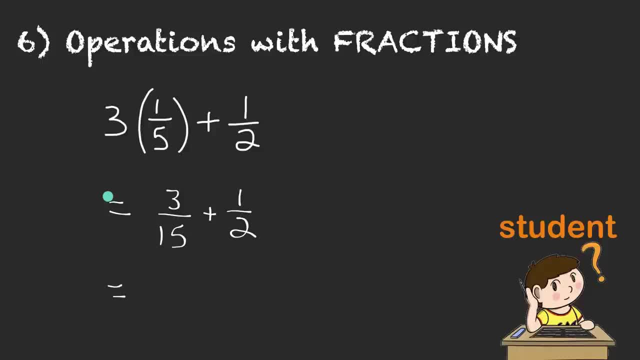 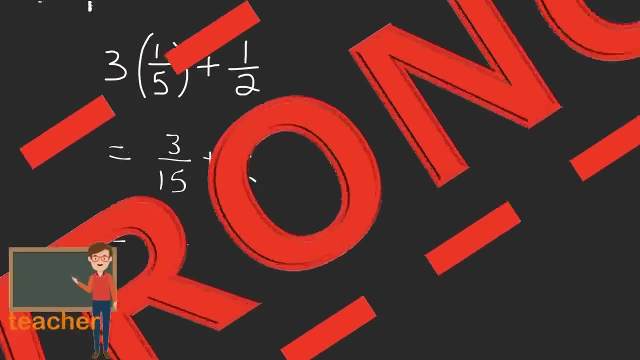 Plus 1 over 2.. And then adding fractions. Okay, so 3 plus 1 is 4.. 15 plus 2 is 17.. 4 over 17.. I think that's good. So you've made a couple mistakes with fraction rules here, The first of which 3 times a. 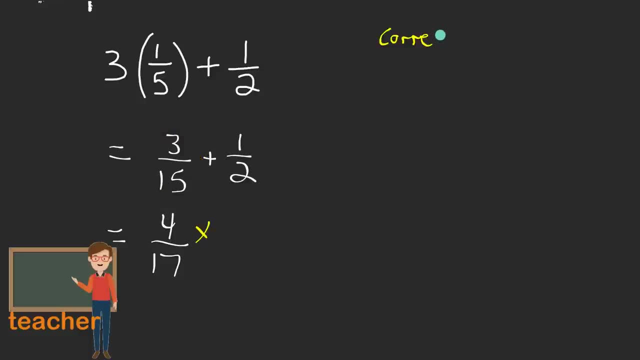 fifth isn't 3 15ths. Let me show you how you can avoid making that mistake of thinking. you multiply a constant into the numerator and denominator, right? It only multiplies by the numerator. Let me show you why. So you can think of that 3, anytime you have a whole number and you're 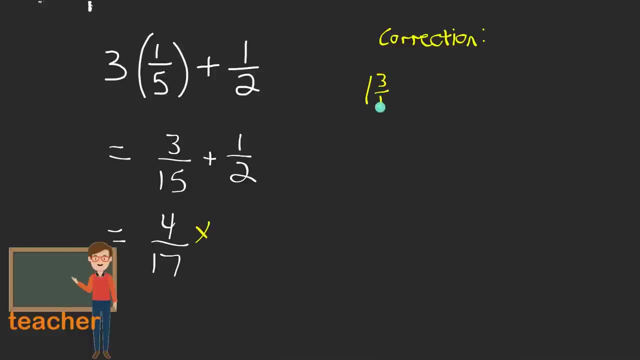 working with fractions. I find it helps a lot if people rewrite that whole number as a fraction over 1.. So that's 3.. Think of it as a 3 over 1.. So I've got 3 over 1 times 1 over 5. And when multiplying fractions you multiply the. 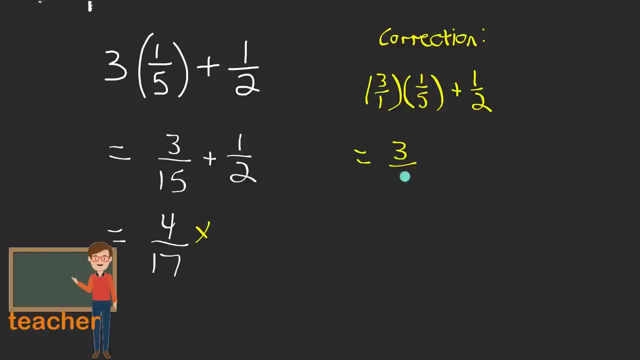 numerators: 3 times 1 is 3. And multiply the denominators 1 times 5 is 5.. So the correct product of the first two is 3 over 5.. The 3 just gets multiplied by the numerator. And when adding fractions, do not forget to get a common denominator, One fraction. 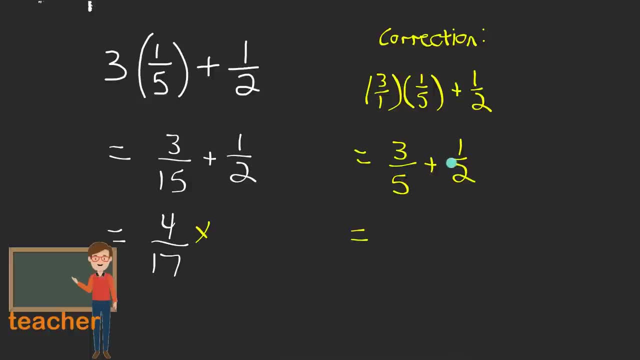 has a denominator of 5, the other a denominator of 2.. A common denominator between those two would be the product of them 10.. So I'll make this one be 10 by multiplying top and bottom by 2.. And this one be 10 by. 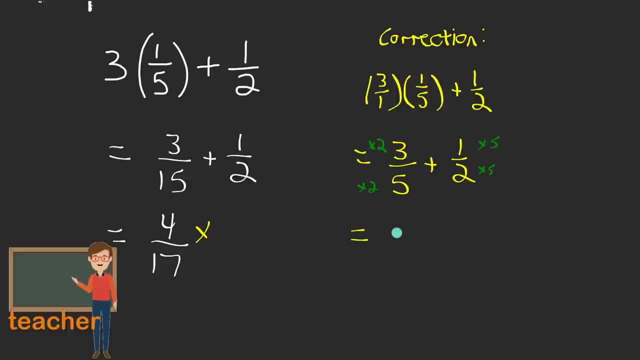 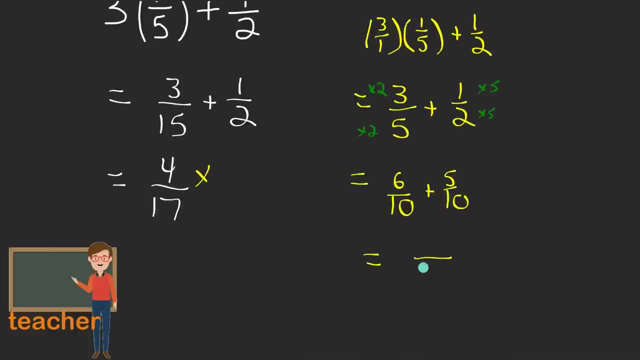 multiplying top and bottom by 5. And that gives me 6 over 10 plus 5 over 10.. And when adding fractions, you keep the common denominator. Don't add the denominators like you did over here. You keep the common denominator. 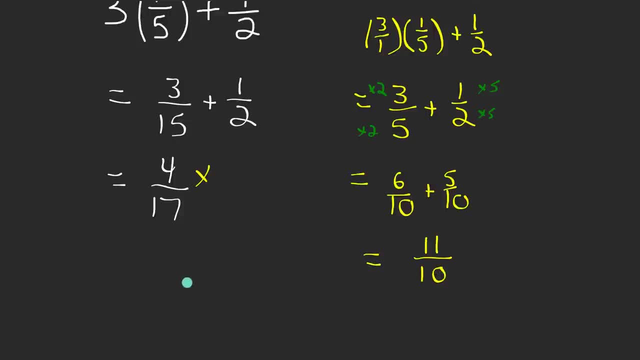 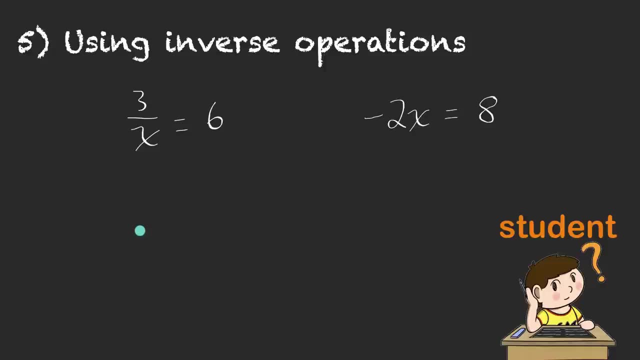 and just add the numerator 6 plus 5, 11.. Okay, I remember my teacher saying I have to do With the opposite operation, to move a term between sides of the equation. Okay, on the left I see a 3.. So when I move it to the right, I think I'm going to divide by 3, which? 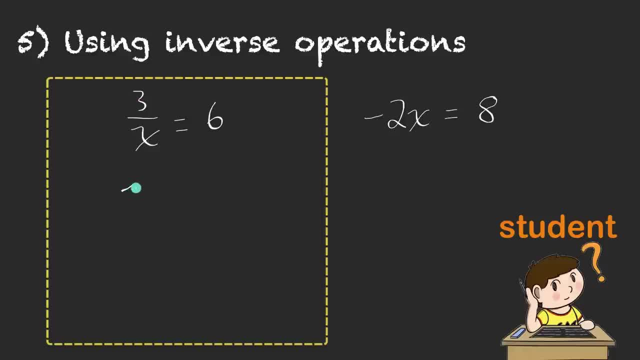 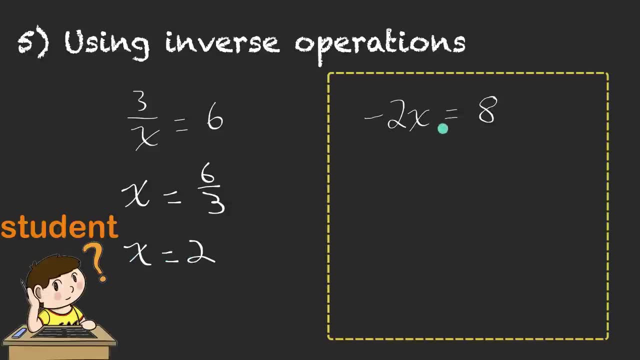 means okay, the 3 is gone from the left, which means I just have the x left And on the right I've got 6 over 3, which is 2.. Oh, this equation over here. negative 2 times x equals 8.. The opposite of multiplying by. 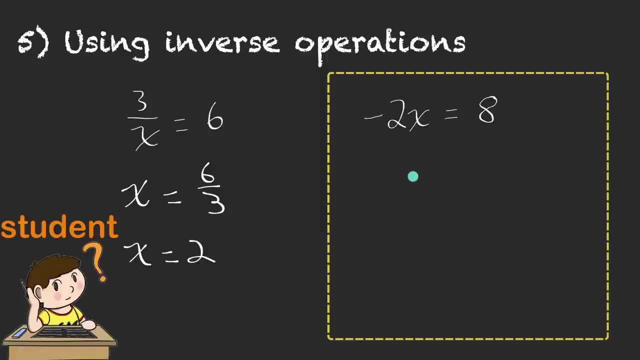 negative 2.. Well, the opposite of negative 2 would be positive 2, and the opposite of multiplying is dividing, so I would divide by positive 2.. So I get x equals 8 over 2,, x equals 4.. 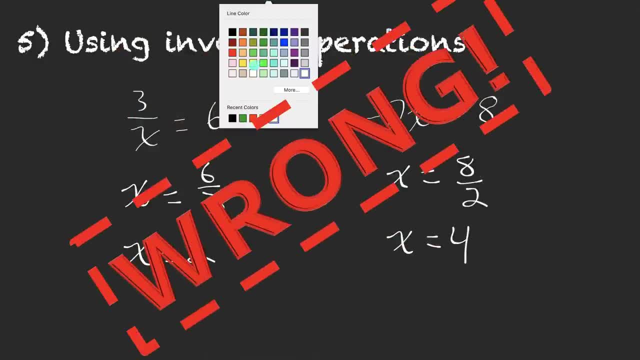 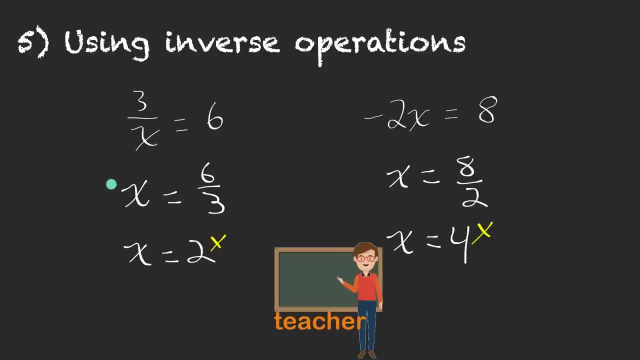 There we go. both of those done, So you're right. you do have to do inverse operations to isolate a variable. It's just you chose the wrong operation so you got incorrect answers. And don't forget, you can check to see if your answers are right by plugging them into the original equation. 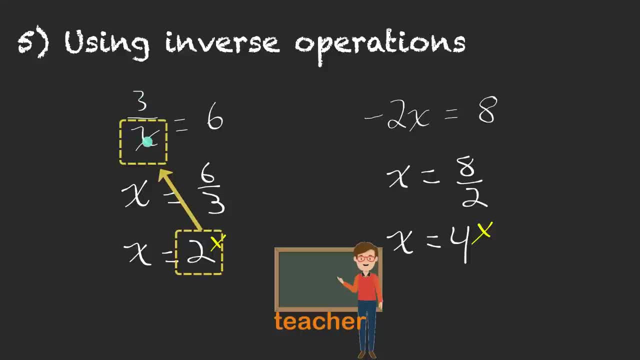 If I plug 2 in for x into the original equation, I get 2.. So I'm going to plug 2 in for x into the original equation. If I plug 2 in for x into the first equation, 3 divided by 2 is in 6.. If I plug 4 in for 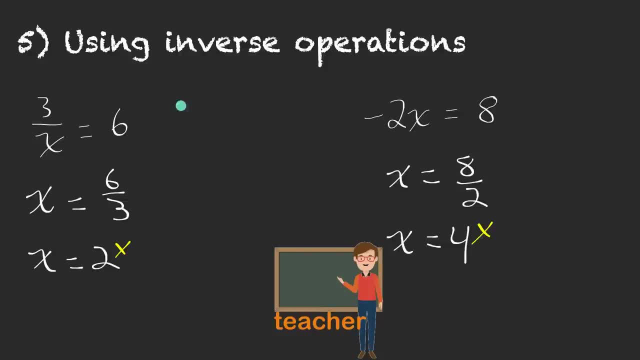 x into the second equation. negative 2 times 4 is not 8.. Alright, let me show you how to correct the first one. To avoid making this mistake, I think you should try and approach it from more of the balanced method when solving equations. 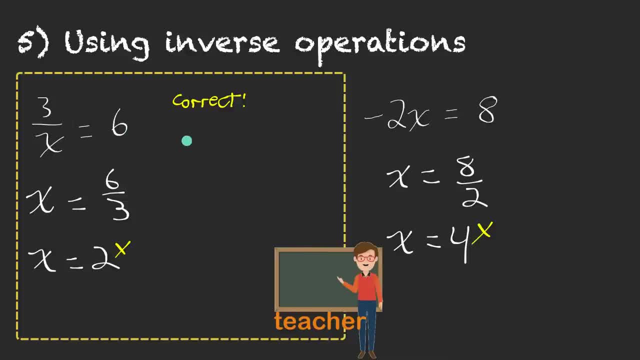 So whatever you do to one side, do it to the other side. So when your variable's in the denominator, let's multiply both sides of the equation by that variable to get it out of the denominator. So x times 3 over x equals 6 times x. 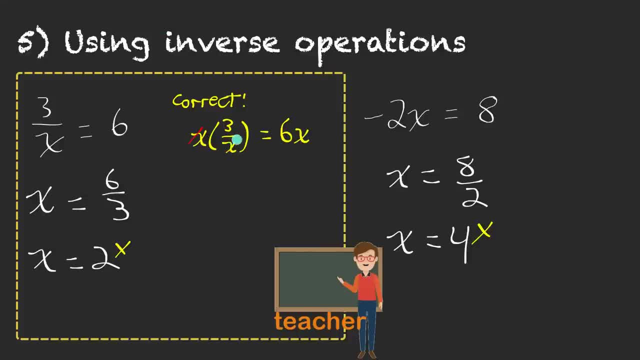 So I just multiply both sides by x. And the reason why I did that is because now we have x over x on the left, which cancel out, and we've got 3 equals 6x. Then divide both sides by 6, and I get a half equals x. And if we check that in the original equation, 3 divided. 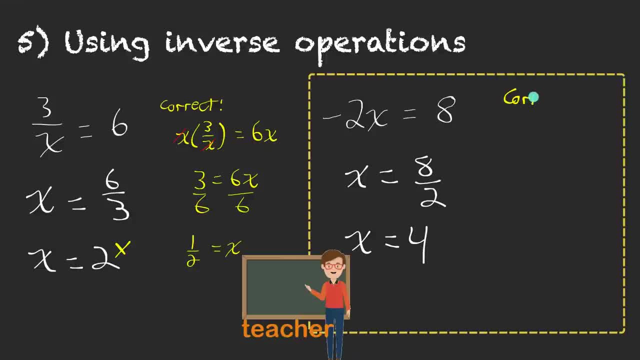 by a half is 6.. Alright, let's correct this one. I understand your thinking here, but if we divided both sides by 2, that doesn't cancel out this negative 2.. Negative 2 divided by 2 is negative 1,. 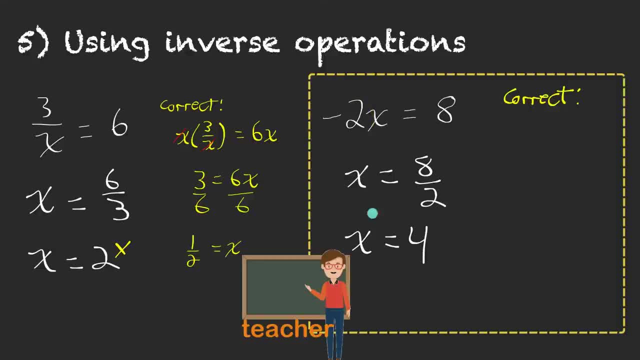 so we'd have negative x equals 4.. What we should do instead is to the original equation: divide both sides by negative 2.. The opposite of multiplying by negative 2 is dividing by negative 2.. And you can see why: because these factors of negative 2 cancel out leaving 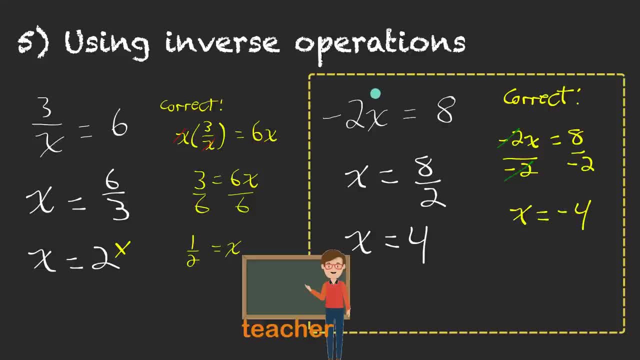 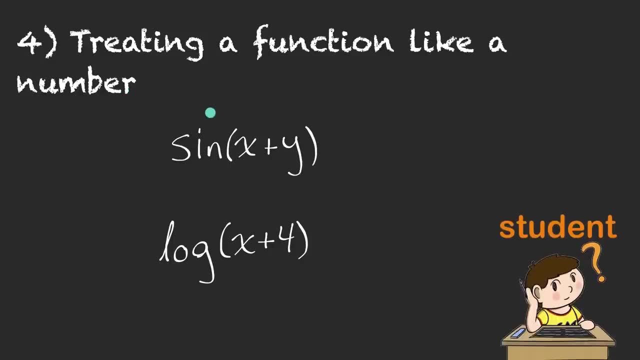 us with x equals negative 4.. And if we check that in the original equation negative 2 times negative 4 is positive 8.. Oh I love it when these easy distributive properties work. I know how to do distributive property. I can just multiply these right into there. 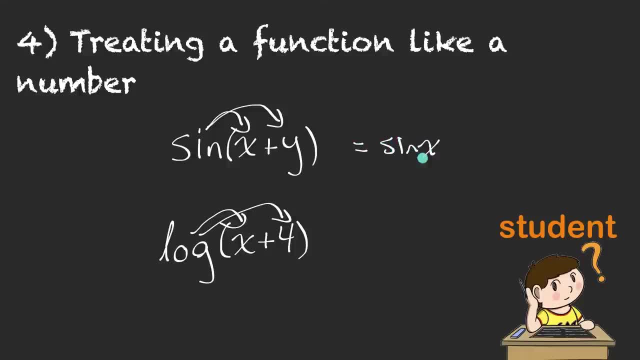 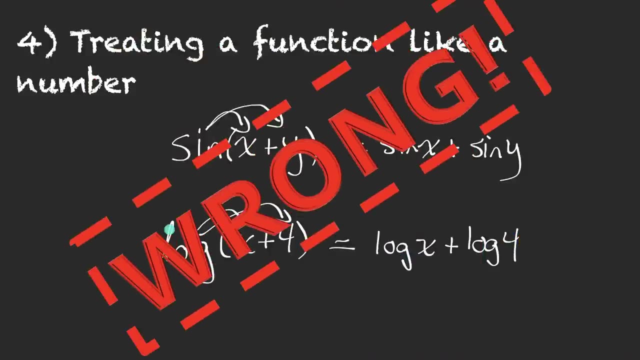 Sine times x plus y. Well, that's just sine times x plus sine times y. And same with log Log times x plus 4?? Well, that's just log times x plus log times 4.. So both of these are incorrect. 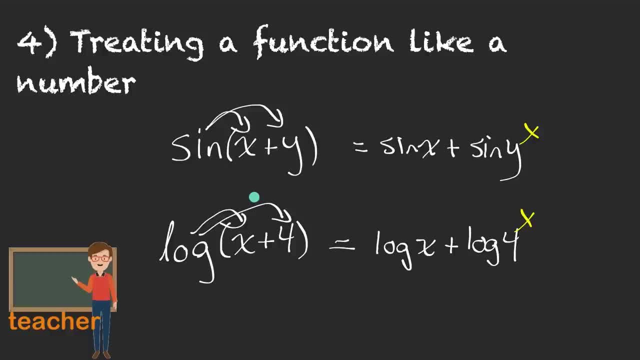 It's a super common mistake to think that sine and log can be treated like numbers and distribute them into their own arguments. Sine and log are functions, though, not numbers. What we have with both of these aren't a product of things. It's not sine, times x plus y and 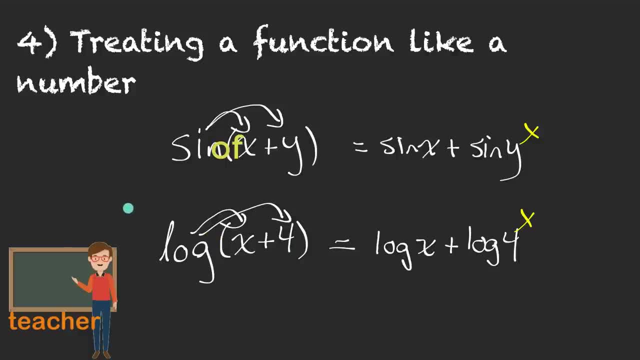 log times x plus 4.. It's sine of x plus y and log of x plus 4.. You can't distribute a function into its own argument, So don't try and treat sine and log as if they were numbers and try and do distributive property. 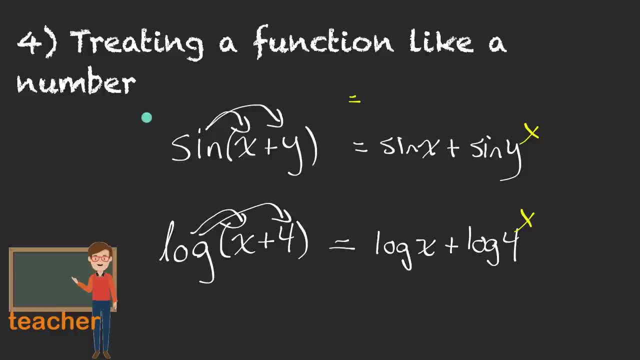 Sine of x plus y. It's actually fairly complicated. There's an identity for that. If you wanted to rewrite sine of the angle x plus y, it's equal to sine x cos y plus cos x, sine y And log of x plus 4?. There's nothing we could do to simplify that. You can't expand a log. 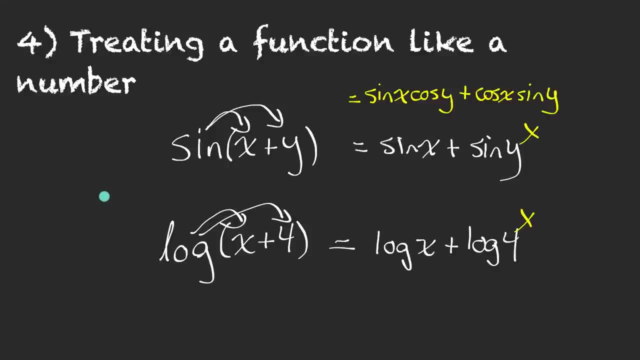 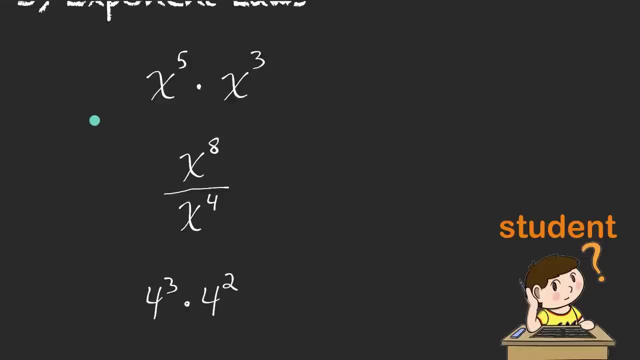 into its own argument. So don't try and do that. Oh, I just have some expressions here to simplify. I remember my exponent laws. Okay, I've got things being multiplied. I know how to multiply, Oh, I think I remember. Okay, you leave the. 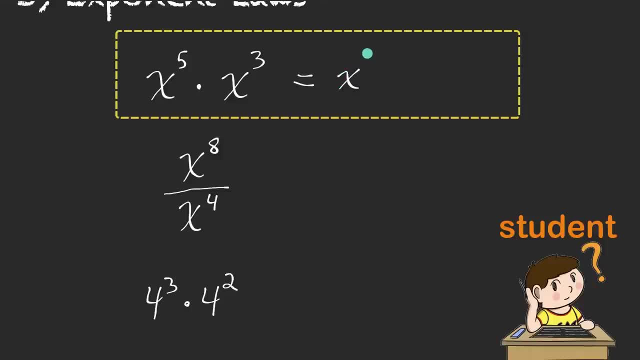 base, yeah, And they're being multiplied 5 times 3, 15.. This next one: Okay, this time the powers are being divided, So I keep the base and 8 divided by 4, 2.. And my last one: 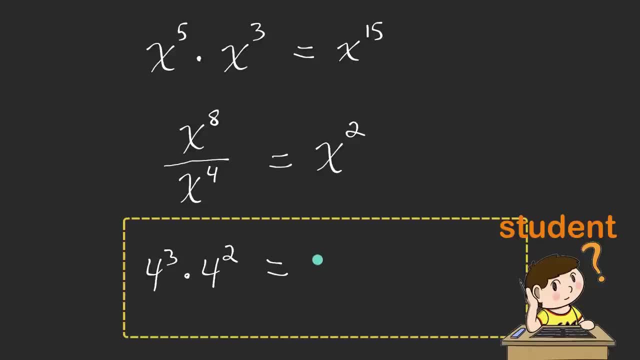 this one. here they're being multiplied. Oh, 4 times 4,, that's 16.. Okay, so my base is 16.. And then I think I remember something about when multiplying powers you, I think you add the exponents 3 plus 2, 5.. 16 to the 5.. Good, 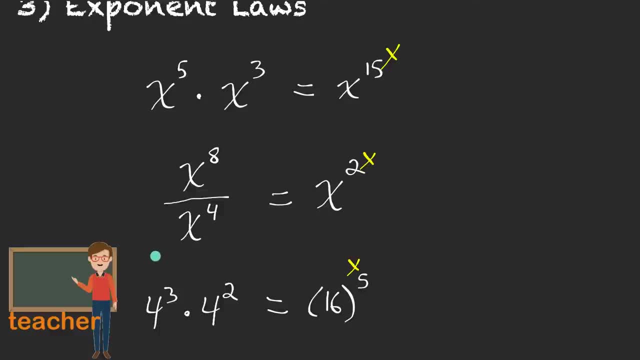 Okay, so all three of these are incorrect. Let's start by looking at the first one. So we do have powers of x Being multiplied together, and when you're multiplying powers at the same base, you keep that base of x, But you add the exponents: 5 plus 3 is 8.. So we'd have x to the 8.. And 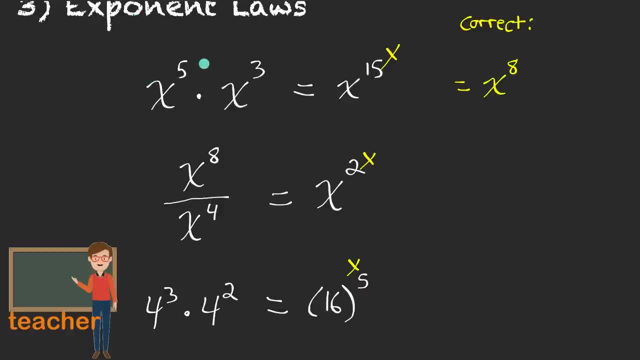 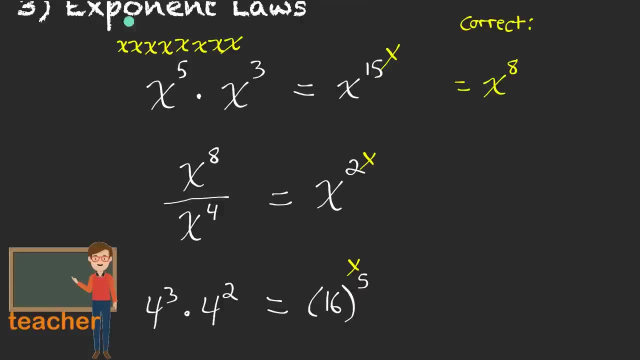 there being multiplied by x, you can see that x to the 5 is x times x times x times x. And if you look at the second one, dividing powers with the same base- yes, you keep the same base. you did that well, But we have to subtract the exponents, not divide them. 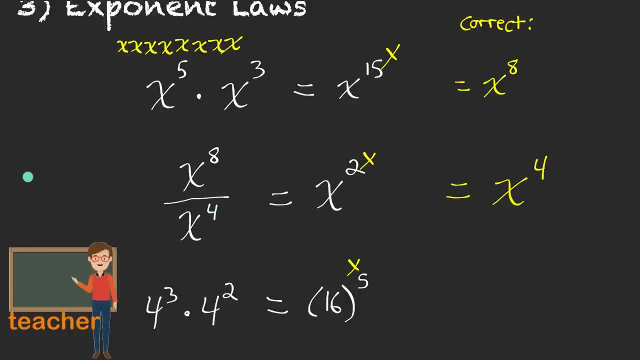 8 minus 4, 4.. And if you want to see why, write it out. So we have 8 factors of x divided by 4 factors of x And you notice that four pairs will cancel out One pair, two pairs. 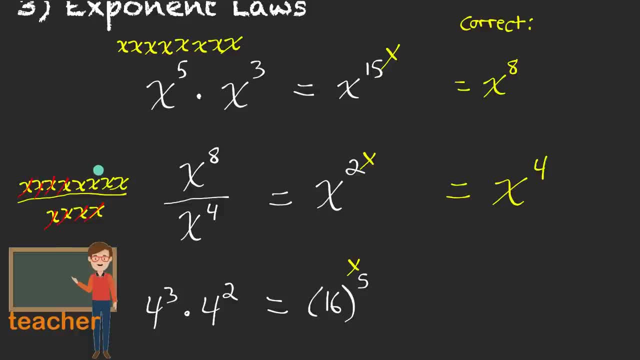 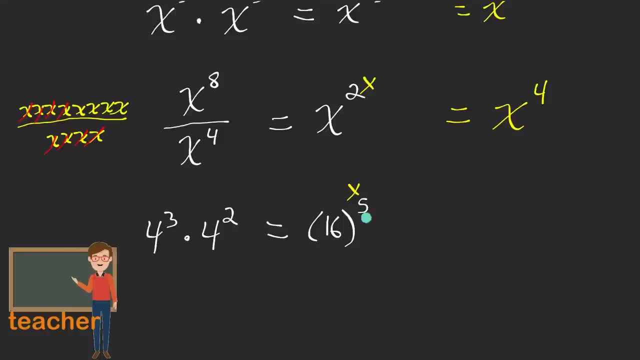 three, four. So what do we have left In the numerator? we have four factors of x, Hence x to the 4.. Okay, the last one was so close Multiplying powers to the same base. Yes, you do add the. 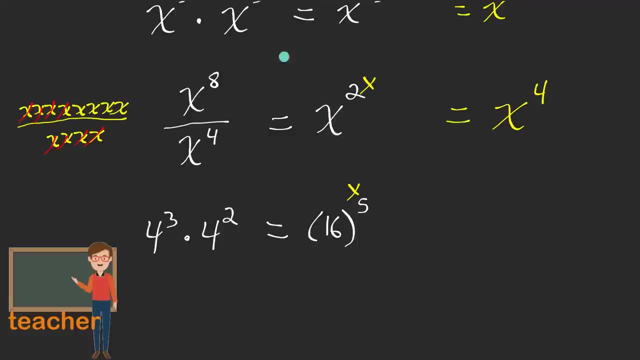 exponents. The exponent is 5.. But you forgot what you did up here. You keep the base the same. It should be 4 to the power of 5.. You don't multiply the bases together. You keep the base the same and add the exponents. 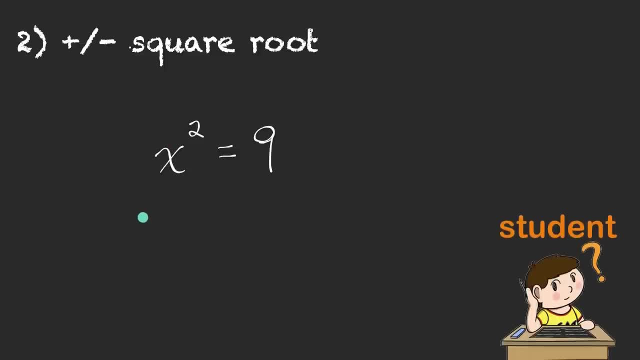 Oh, solving an equation Easy, Easy. Inverse of squaring is square rooting. So on the other side, if I move the squared, it becomes square root. I get the square root of 9, which is 3.. And let me check and see. 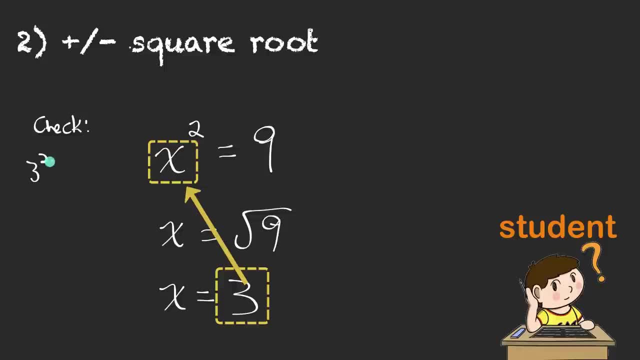 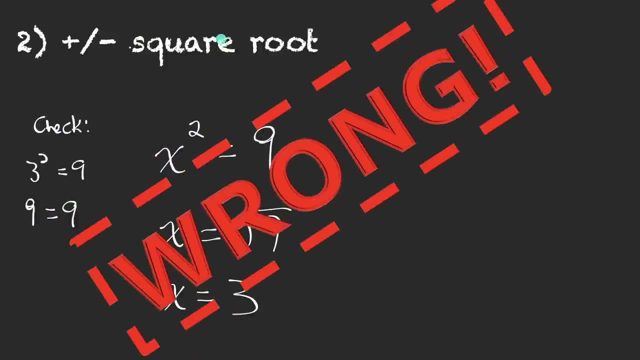 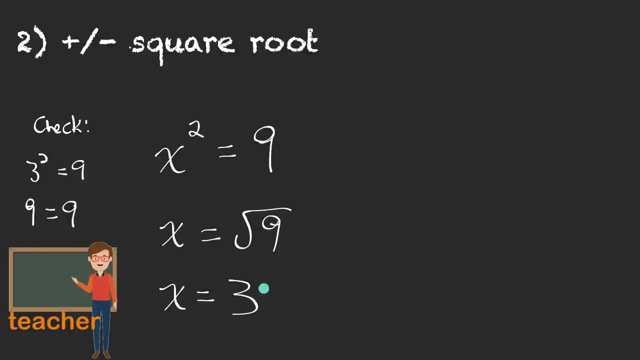 if that's right. If I plug it back in, is 3 squared equal to 9?? Yep, 9 equals 9.. Good, I know I got the right answer this time. Okay, you did get one correct answer for this question. 3 is the correct answer: 3 squared. 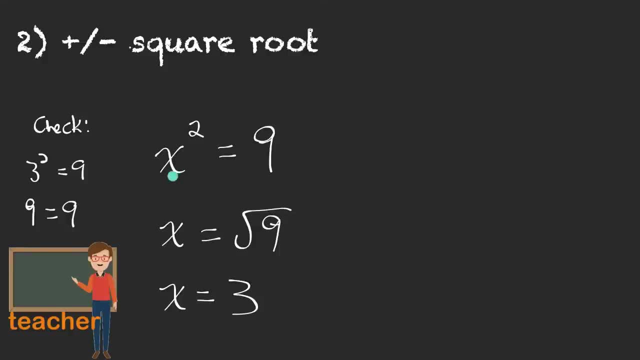 does equal 9.. But it's not the only correct answer. The inverse of squaring is actually plus or minus square rooting. So you should have got plus or minus 3 as your answer. Right, If you square negative 3, you also get 9.. So that's also a solution to the equation. 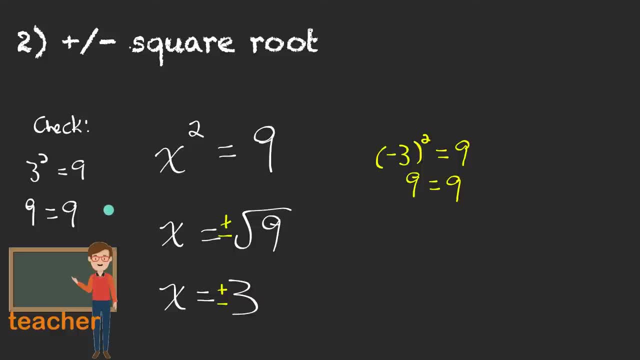 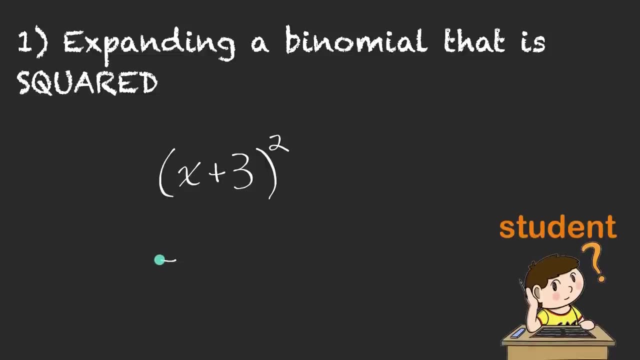 So this is just an example how some equations can have more than one answer. So make sure you find all answers that satisfy an equation- This one. Okay, the base of my power is being squared. I can just put this- exponent 2, on the x and the 3.. So I've got x squared plus 3 squared. 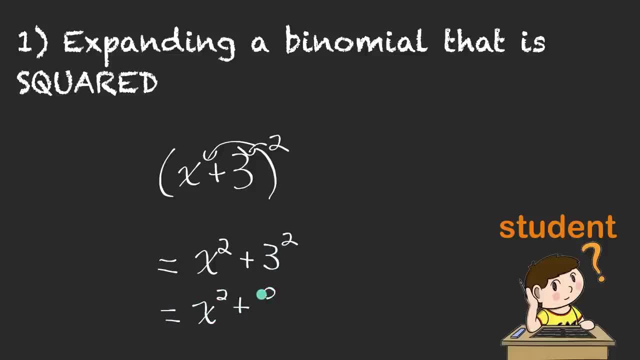 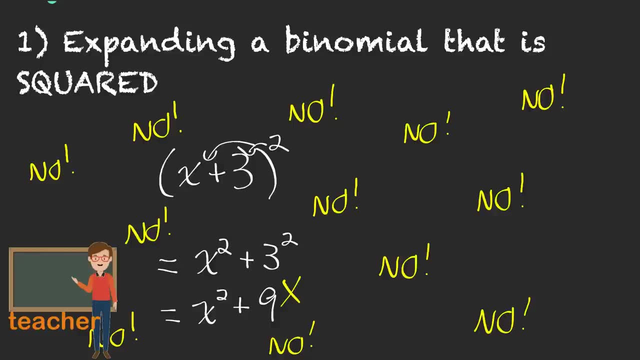 Oh, and I'll make sure I simplify that: 3 squared is 9.. Perfect, Okay, so this is incorrect. You can't take the exponent and put it on both terms in the base if in the base, the terms are being added or subtracted. This is the most common mistake. 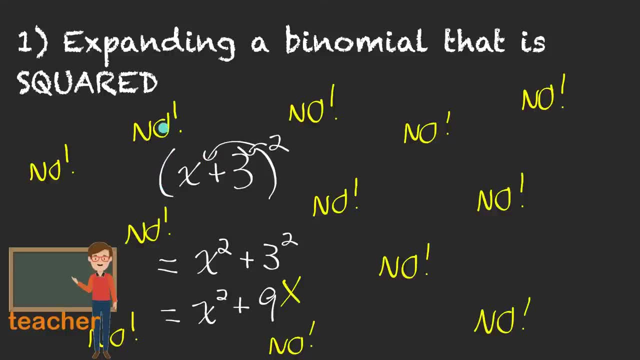 made in all of the high school math courses. So try never to make this mistake. Look at the base of your power. If it's terms being added or subtracted, you can't just put the exponent on both. So how can you not make this mistake? Rewrite that x plus 3 squared. 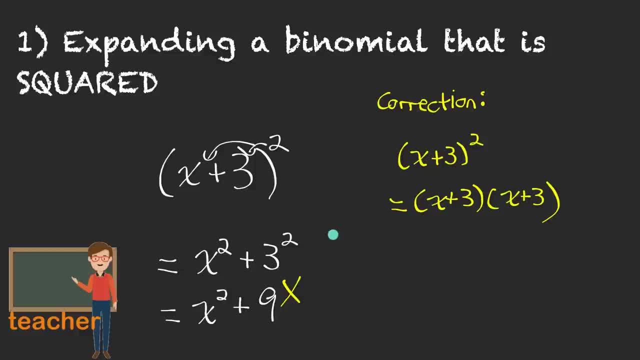 as x plus 3 times x plus 3.. That way you can see. what you need to do is you need to find the product of these two by FOILing it. I need to do the product of the x's plus the product of x times 3 plus. 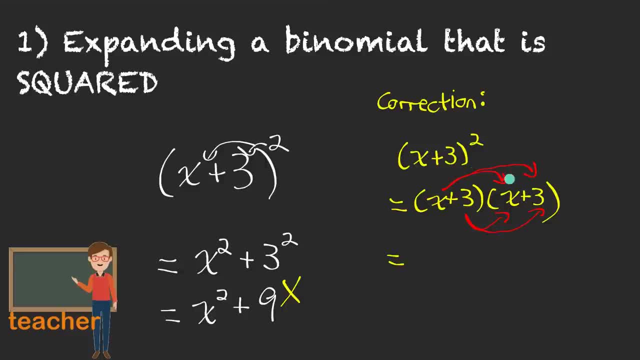 x plus the product of 3 times 3, which gives me x times x is x squared plus x times 3 is 3x plus 3 times x is another. 3x plus 3 times 3 is 9.. So, yes, there is an x squared and. 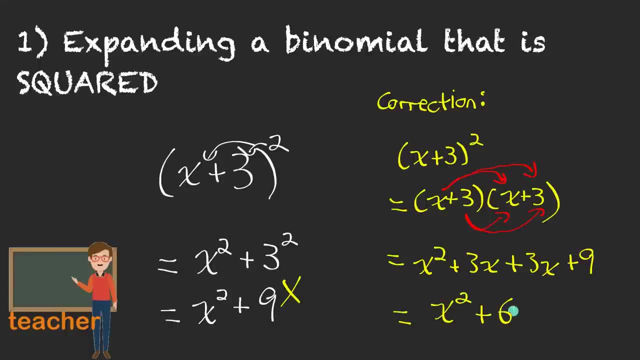 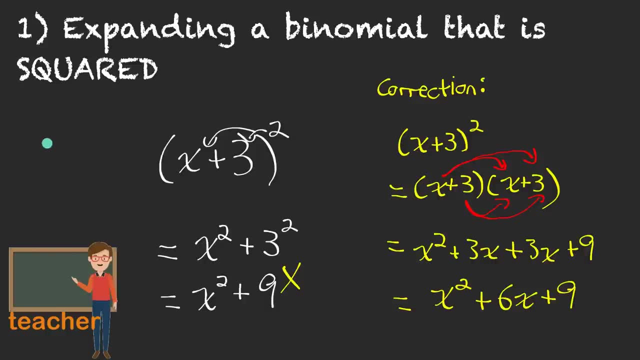 a 9,, but there's also a middle term. It's x squared plus 6x plus 9.. I think maybe what you were thinking of when you tried to do this, like, let's say, it was 3 times x squared. yes, there is an exponent rule for that. 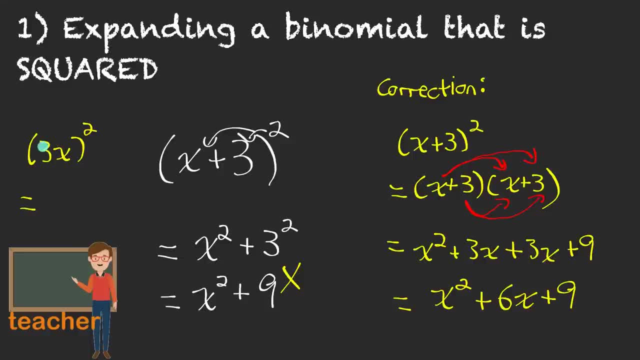 If the base of the power is a product of two numbers, we can put the exponent on both of the factors of the base. So, yes, this would equal 3 squared times x squared, which is 9x squared. So in that case you can.